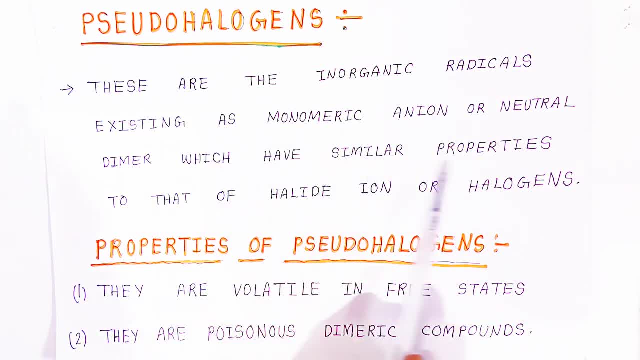 Monomeric anions are neutral dimers which have similar properties, so that of halide ions, It is mostly similar to what Halide ions. that is why it is called as what Pseudo halogens. It is not a halogens, but it is look like a halide ions. that is why it is called as what Pseudo halogens. 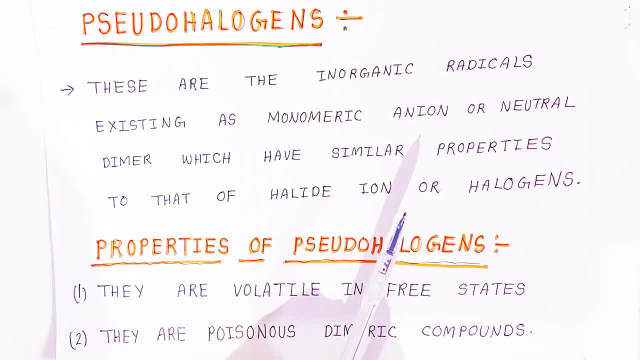 Understanding students. So here I have written halogens. It is asked in examinations: what are the pseudo halogens You have to write? these are the inorganic radicals existing as monomeric anion or neutral dimer. You can also say what Neutral dimer which have similar properties. 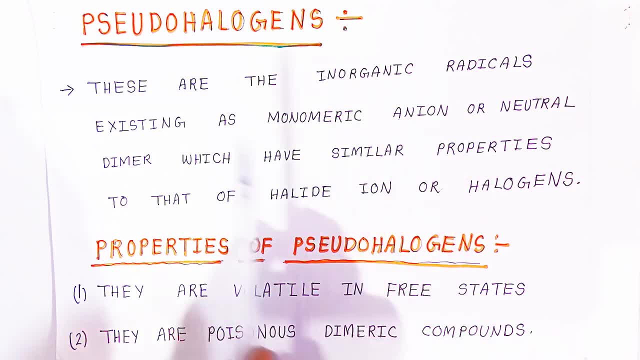 like halide ions and halogens, but they are not actual halogens. That is why it is called as what, Pseudo halogens. Now, students, we are going to see the properties of pseudo halogens. First of all, what are the properties they are having? First property is they are volatile in. 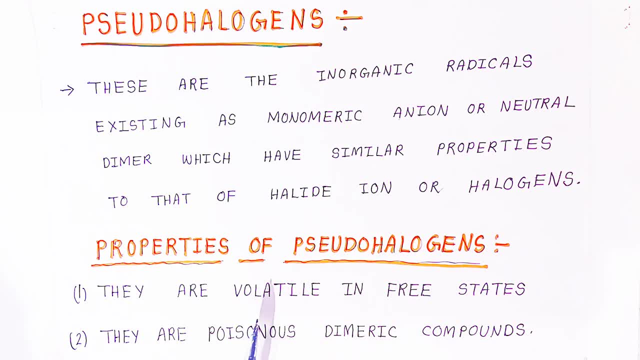 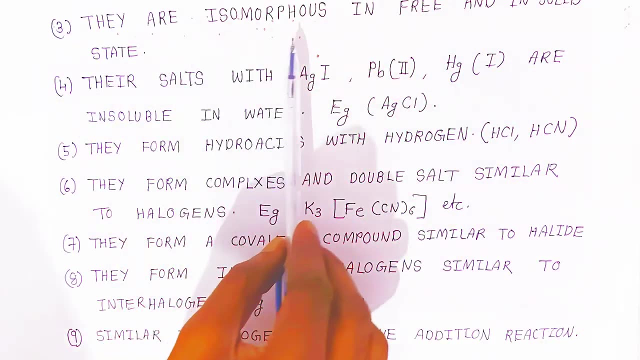 free state. if they are present, free state, they are always. they will volatile Understanding. So they are what Volatile in free state? They are poisonous dimeric compounds. They are very, very poisonous dimeric compounds. They are isomorphous. in free and in solid state They are 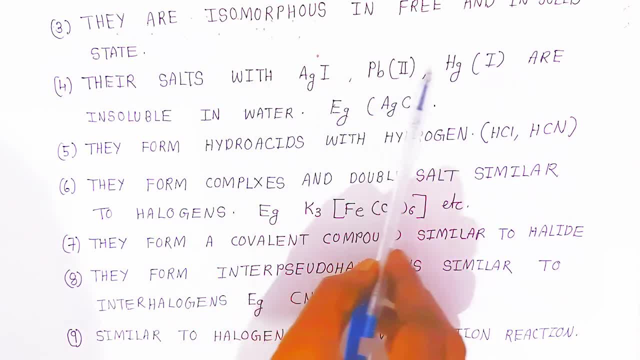 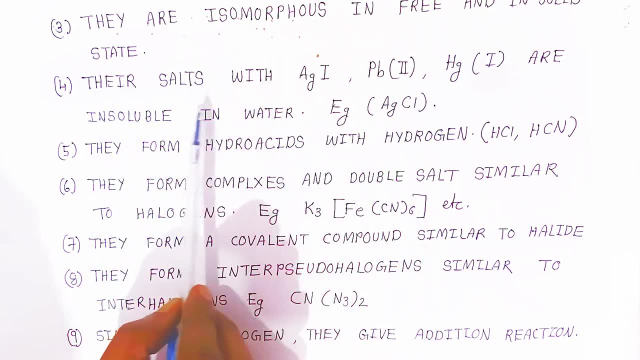 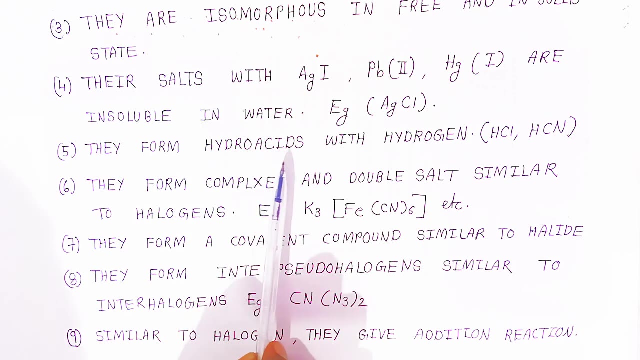 salts with silver iodide le2 plus mercury posion plus are insoluble in water, say for example silver chloride. their salts with silver iodide lead 2 plus mercury 1 plus are insoluble in water. they form hydro acids. they are, they are. 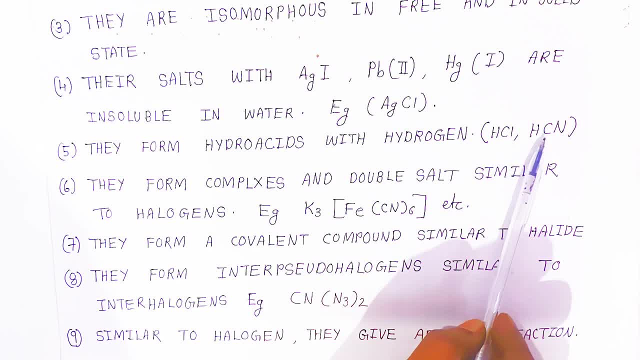 from what hydro acid with hydrogen say, for example, acl, hydrogen cyanide, hydrogen cyanide. they form complexes and double salt similar to halogens. so these are the what there? it is a complex salt. they form a covalent compound similar to halide. they are also forming what? 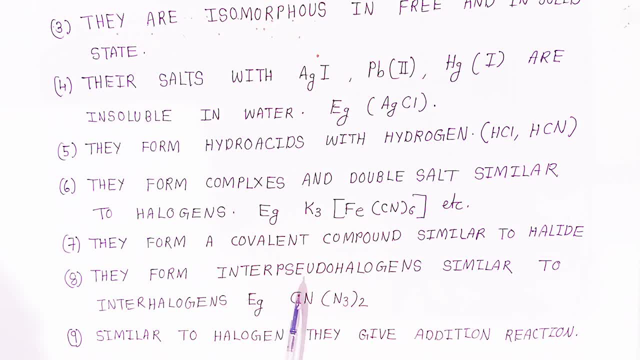 covalent compounds like a halide. they form inter pseudo halogens similar to the inter halogens. understanding students: they are also forming what inter pseudo halogens similar here the example: students i have given cyanogen, cyanide with nitride, similar to halogens. they give addition. 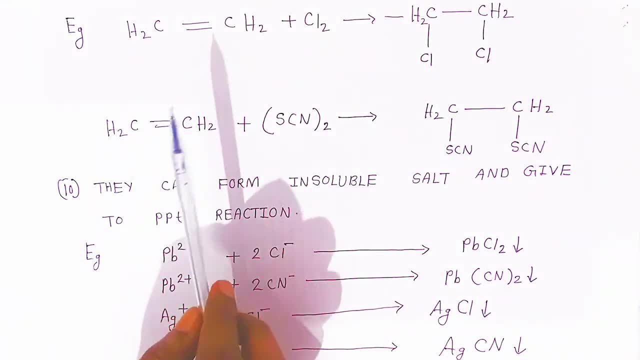 reaction. they are also giving the addition reaction here, students, i have given it is a what ethene combines with chlorine gas. it is forming what? one, two dichloro ethene. now what happens, students? these when combined with thiocyanide? it is combining. like this, the double bond will become one single bond and these two cyanide.